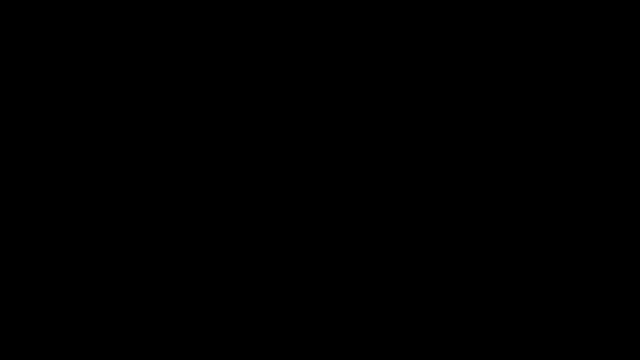 In this video, we're going to focus on reactions associated with amines. So let's start with butyl bromide or 1-bromobutane and let's react it with excess ammonia. So what's going to be the product of this reaction? Ammonia is going to act as a nucleophile in this reaction, attacking the carbon from the back, expelling the leaving group. 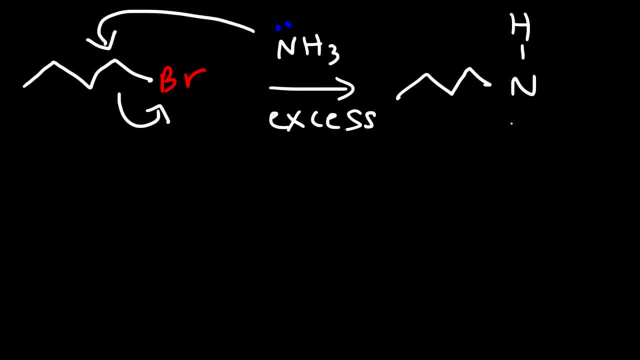 And so this is going to be an SN2 reaction, And so right now the nitrogen atom has a positive charge, since it has four bonds. Now another NH3 molecule is going to remove a hydrogen, And so right now we have butylamine, And so that's the simple way in which we can make an amine. 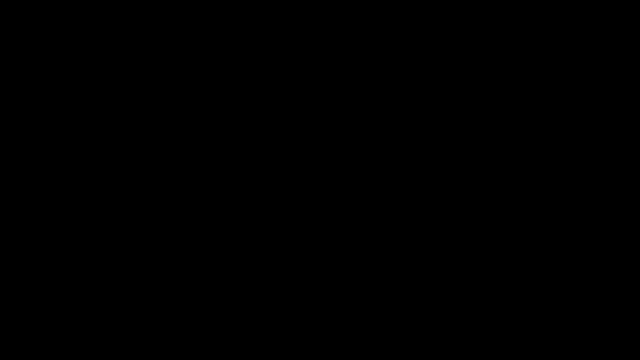 Now there are two ways to make an amine. Now there are some problems with that reaction, particularly exhaustive methylation, For example. let's say, if we were to react ammonia with methyl bromide, The ammonia molecule can attack the methyl group, kicking out the leaving group, And so we're going to get CH3 and NH3. 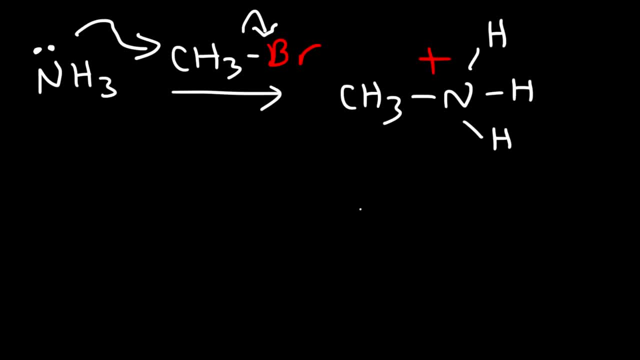 Now, in the next step, Another NH3 molecule is going to basically remove a hydrogen, And so now what we have is methyl amine. Now this will react with methyl bromide again, And so we can add another methyl group to the nitrogen atom. 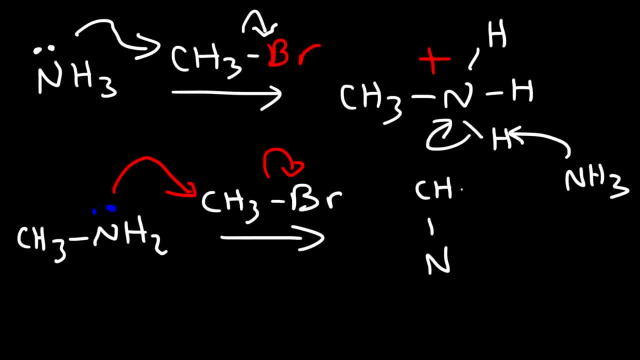 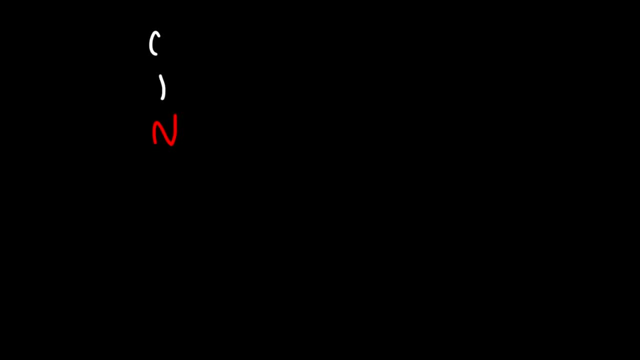 And so right now the nitrogen atom has two methyl groups And two hydrogen atoms, So now it carries a positive charge And this process can repeat until the nitrogen atom has four methyl groups, And so this is called exhaustive methylation. So we need to find better ways to produce an amine, because the nitrogen could attack an alkyl halide multiple times. 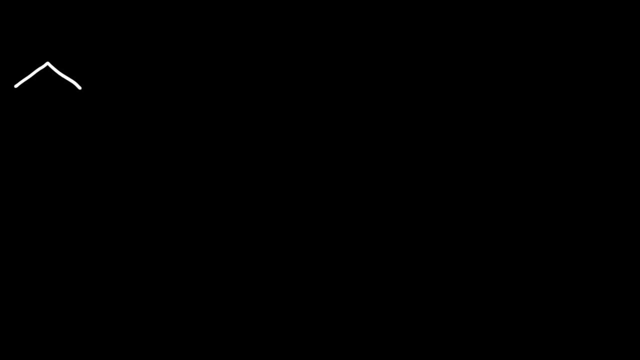 Another way in which we could synthesize an amine is by reacting an alkyl halide with sodium azide, NaN3.. So the N3- ion is the nucleophile in this reaction, And so in an SN2 reaction it's going to displace the bromine group. 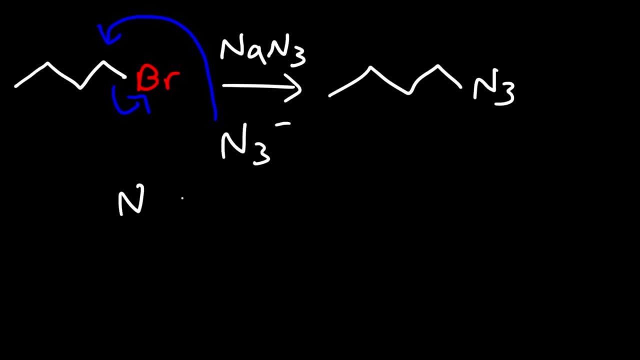 And so we're going to get this. Now the N3 ion looks like this: In the middle we have a nitrogen, We have a nitrogen with a positive charge, And at the end each nitrogen has two lone pairs, so they both carry a negative charge. 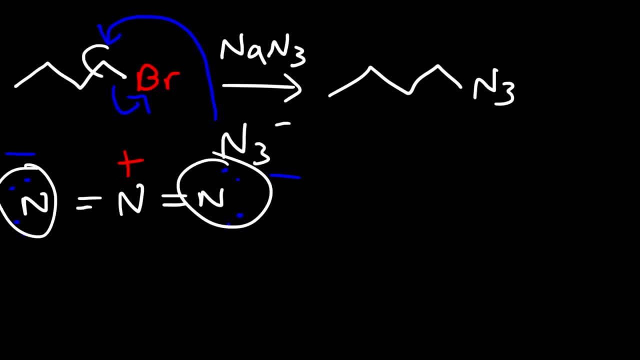 So one of these two nitrogens attacks the carbon atom, And so this structure, this compound, looks like this. So here is the nitrogen with a positive charge. On the left, the nitrogen is neutral Because it has three bonds. On the right, it has a negative charge. 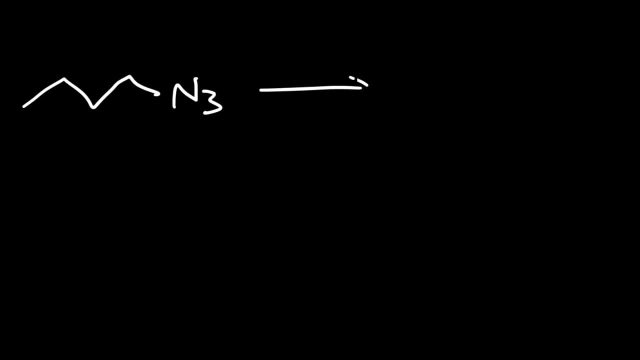 So once we have this compound, we can reduce it using lithium, aluminum hydride, followed by H2O, And we're going to lose two of the three nitrogen atoms, But the last one that remains will be reduced to an amine. 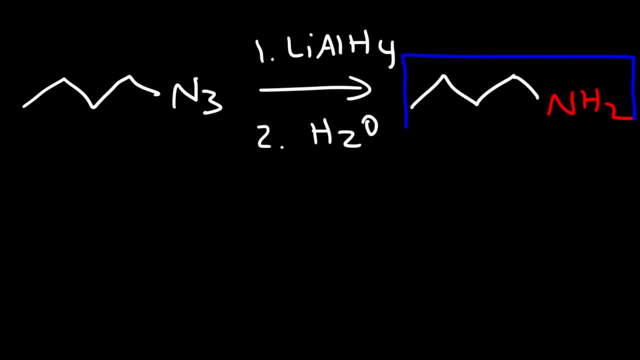 And so that's another way in which we can make An amine from an alkyl halide. Now the next thing that we could do, starting with an alkyl halide, is we can react it with sodium cyanide, And so the cyanide ion is going to be the nucleophile in this reaction. 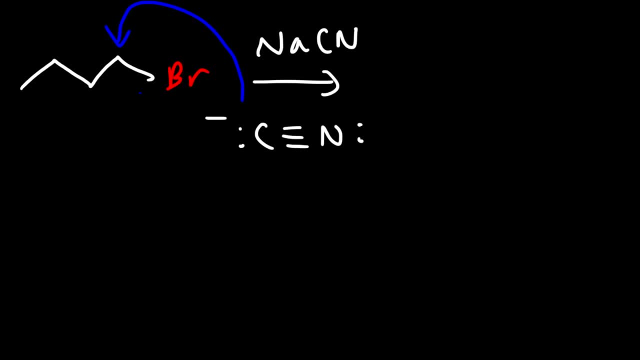 The carbon has the negative charge, And so it attacks the carbon, with the halogen kicking out the leaving group, And so we're going to get a nitrile. Now we can reduce the nitrile into an amine, And so we could use hydrogen gas with a metal catalyst such as nickel. 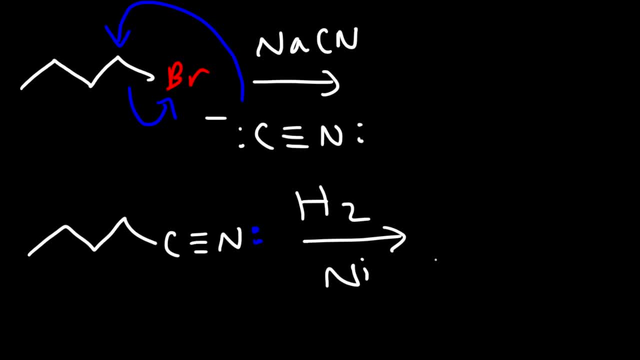 We could also use lithium, aluminum hydride in the first step, followed by H2O, And so what we're going to have is a total of five carbons and an NH2 group. So this is another way to convert an alkyl halide into an amine by 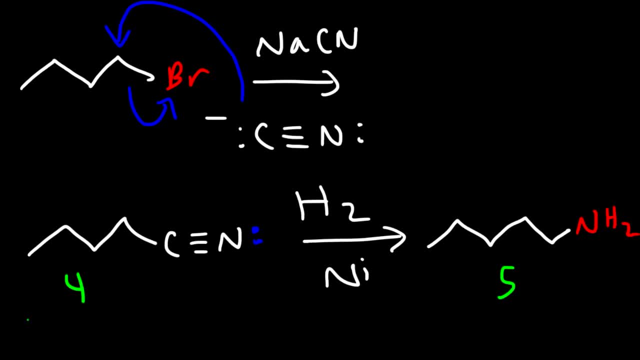 The addition of a carbon atom. So before we had four carbon atoms, but now we have a total of five. Another way in which we can make a primary amine is by using the Gabriel synthesis reaction, And so in this reaction we're going to start with this compound which is called thalamide. 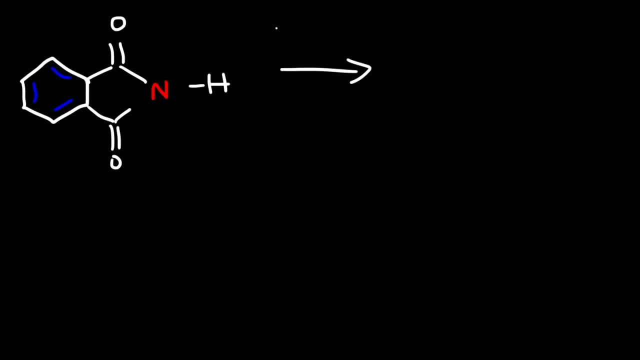 And in the first step, we're going to react it. We're going to react it with potassium hydroxide, And so this is to deprotonate the hydrogen, put in a negative charge on the nitrogen, which becomes a nucleophile. for the next step, 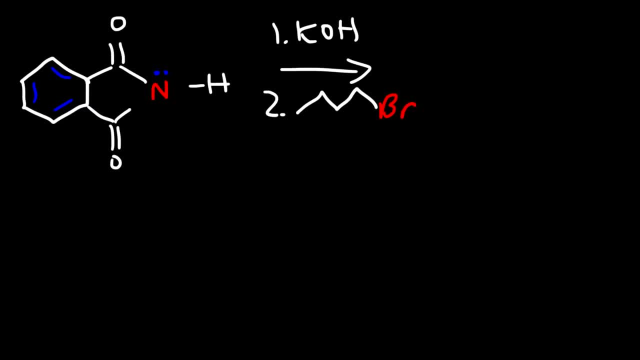 And then we're going to react it with an alkyl halide, attaching the nitrogen to those four carbons. And finally, we're going to use hydrazine. You can write it as N2H4 or H2N-NH2, with heat. 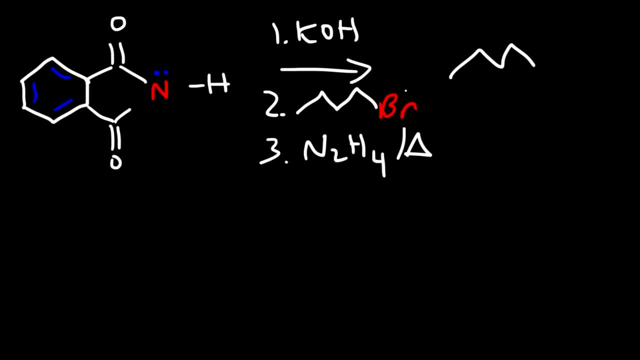 And so what's going to happen is we're going to replace A bromine atom with an NH2 group, So this is going to be the main product. So we have butyl amine, And a side product that we're going to get will look like this: 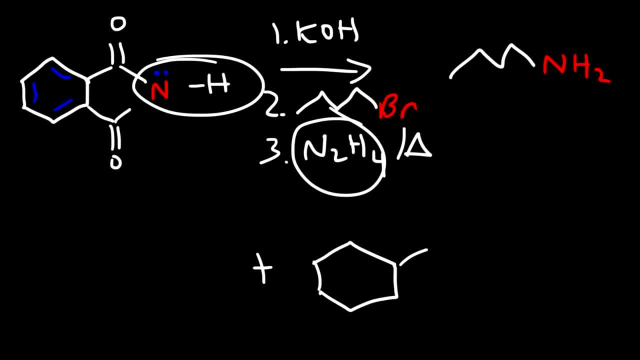 So the hydrazine molecule will replace this NH group, And so this five-atom ring is going to expand into a more stable six-atom ring, And so we're going to get something that looks like this: So that's the other side product for this reaction. 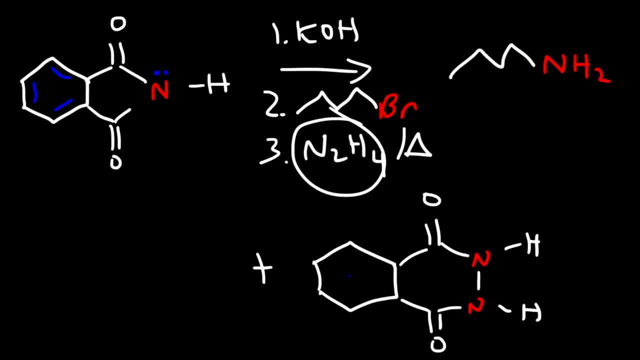 So this is called a thalamide hydrazine. But the purpose of the Gabriel synthesis reaction is to make primary amines. So the first step in the mechanism of this reaction is that the hydroxide ion takes off this hydrogen. 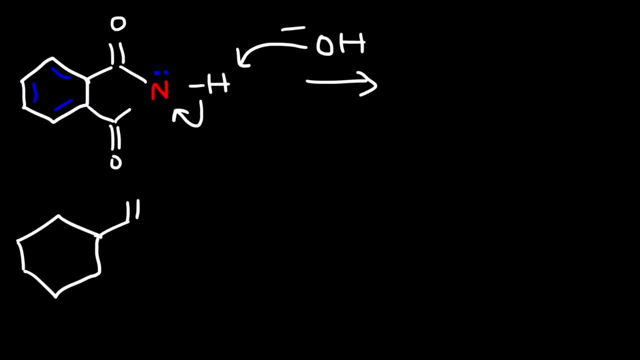 And so we're going to have a negative charge on the nitrogen. But the reason why that hydrogen is relatively acidic is because the conjugate base is stabilized by resonance. So now that the nitrogen atom has two lone pairs, we can draw a resonance structure with the carbonyl group. 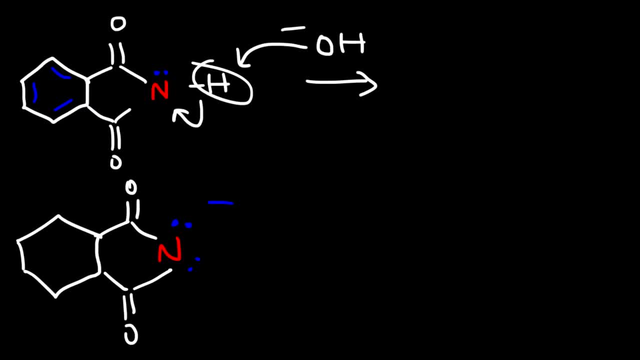 And so that's why this hydrogen is relatively acidic compared to other NH bonds. So now that we have a nucleophilic nitrogen atom, we can now react it with Butobromide, And so it's going to attack the carbon, kicking out the bromine group. 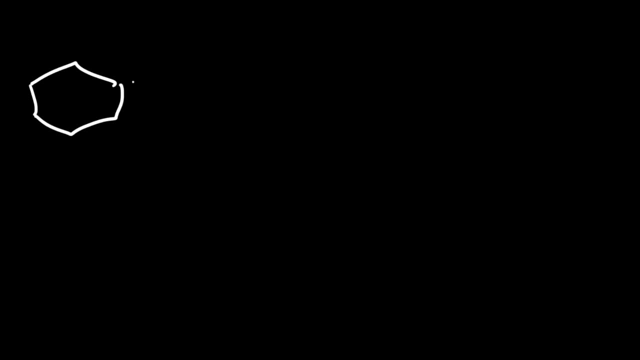 And so right now we have this structure, So we have an N with a butyl group, And once we react it with hydrazine, This will give us the primary amine Plus Thalamide hydrazide which we drew already. 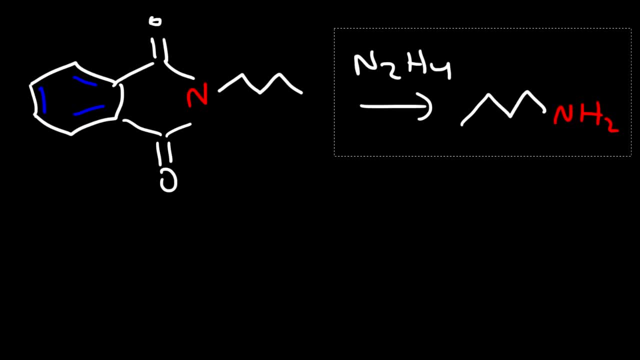 But let's say, instead of reacting it with hydrazine and heat, what if we did something else? What if we react it with H2O plus and heat? What's going to happen? Well, if you have, let's say, an amide and you react it with H2O plus with heat, you can hydrolyze the amide bond. 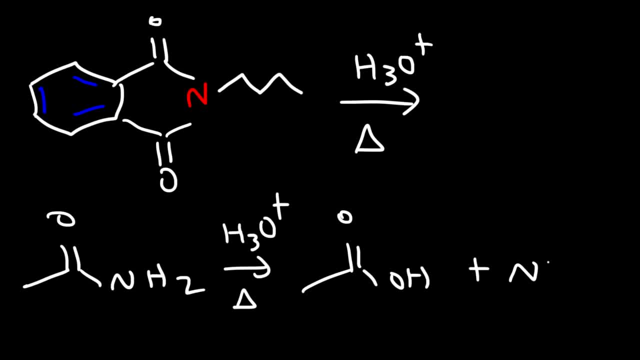 So you're going to get a carbosilic acid And an ammonium ion, So something similar will happen here. So this bond will be hydrolyzed, turning this into a carbosilic acid, And the same is going to happen to this bond. 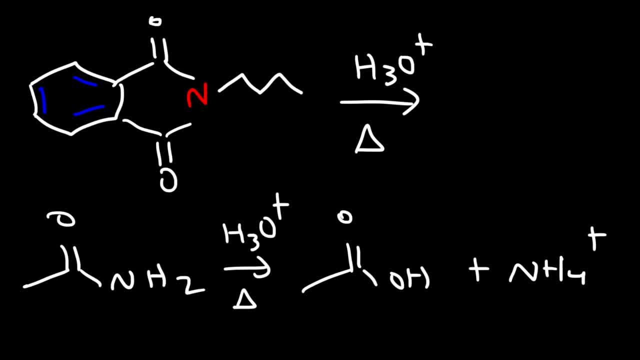 So if we react this with H2O plus and heat in the final step, We're going to get a side product which basically contains a benzene ring with two carbosilic acid Functional groups, And we're going to get our product, but in its protonated form because the solution is acidic. 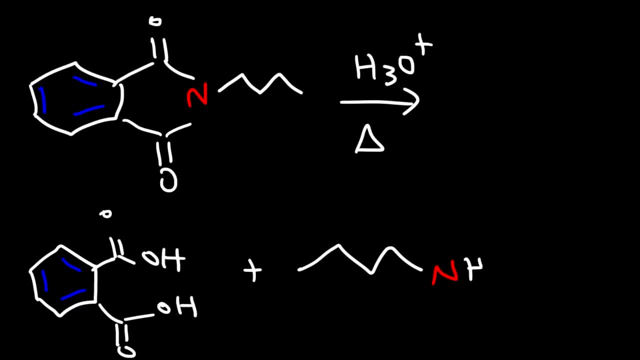 So we're going to get an ammonium ion instead, But we can add some base to this, let's say hydroxide, Just enough to basically remove the hydrogen and turn it to an amine. So If you use H2O plus instead of hydrazine, just know that you're going to get two carbosilic acids on a benzene ring as your side product. 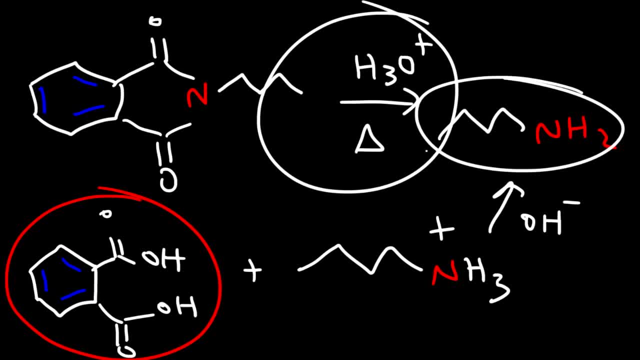 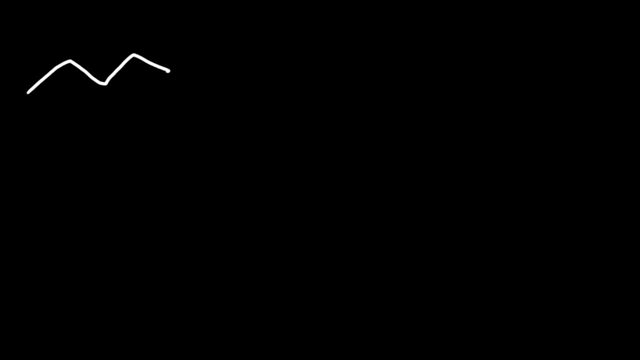 But you could still get the same amine in the end if you basically increase the pH of the solution. Now, let's say, if we have a nitro group on a carbon chain, If we reduce it with iron, metal and hydrochloric acid. 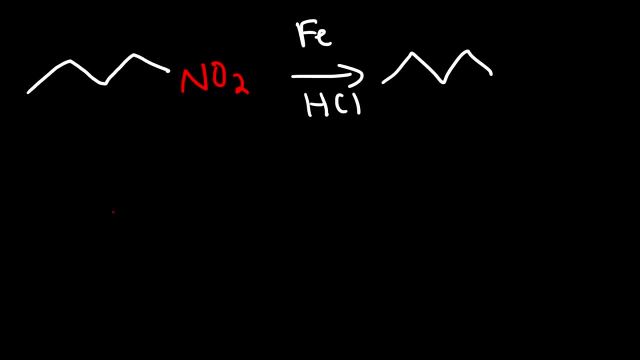 This will turn into an NH3 plus group And then, if we add a base to the solution, we could turn it into an amine. So that's another way in which we can make an amine. It's by converting a nitro group to an NH2 group by reduction. 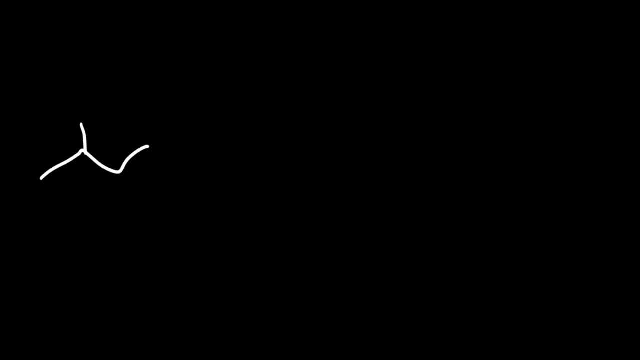 So here's another example. So let's say if the NO2 group was on a secondary carbon? Another way in which we could reduce the NO2 group is by using catalytic hydrogen gas, So hydrogen gas with a metal catalyst, And that's going to turn the NO2 group into an NH2 group. 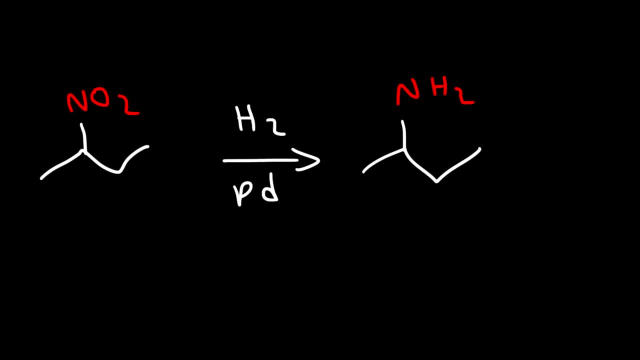 So that's how you can make an amine from a nitro group. Next up, we have a ketone and NH3. What do you think is going to happen if we mix a ketone with ammonia? So what we're going to lose is water. 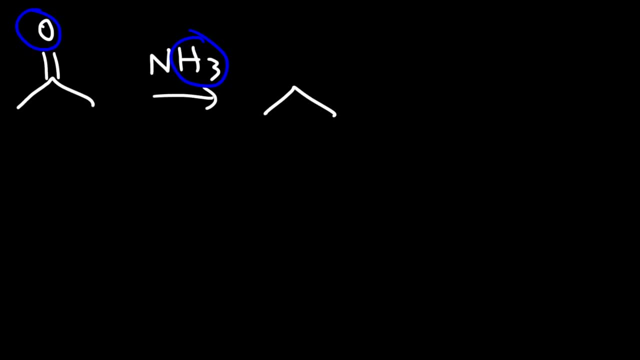 We need to take off two hydrogens and an oxygen, So we'll get water as our side product And then the main product will be an amine which will look like this, So one of the hydrogens will remain. Now, once we have an amine, we could reduce it using sodium cyanoborohydride. 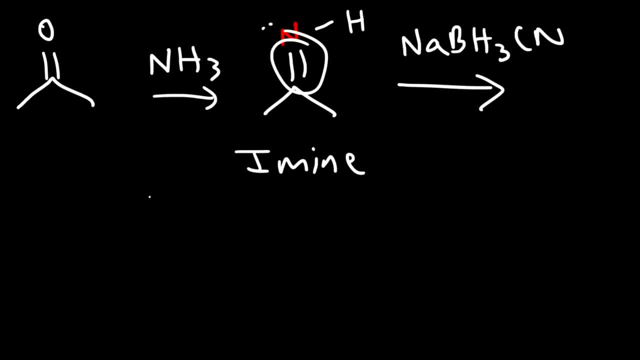 And so it's going to reduce the double bond into a single bond, Converting the amine into a product, A primary amine, which looks like this, Or we can draw it this way: So that's how we can convert a ketone into a primary amine. 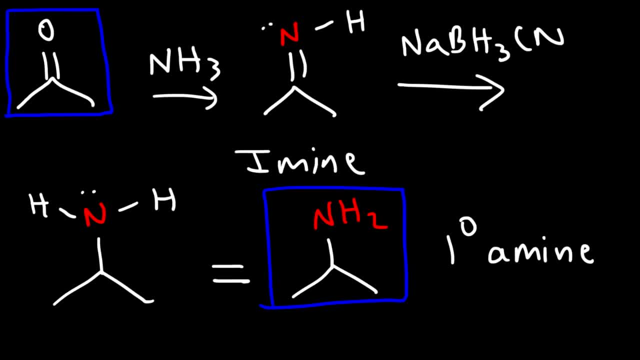 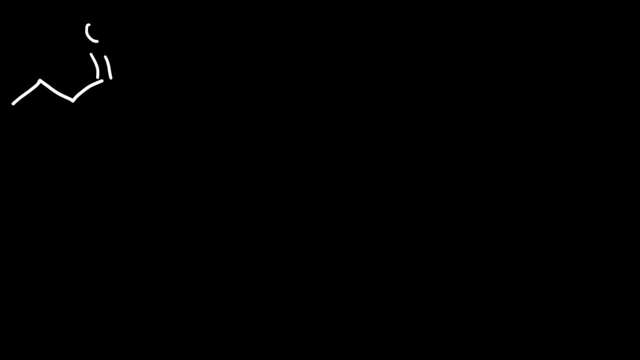 This process is called reductive amination. Now, let's say, if we have an aldehyde or a ketone And we chose to react it with NH3. We can get this product. We're still going to get a primary amine. 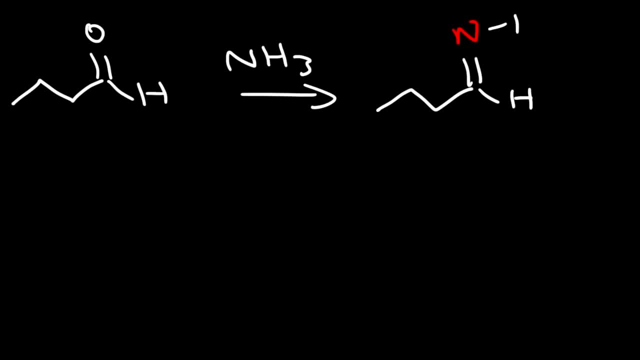 But first we're going to get the imine, Just like before, And then we're going to reduce it using the same reagent, Sodium cyanoborohydride, And so this time the amine is on the end. 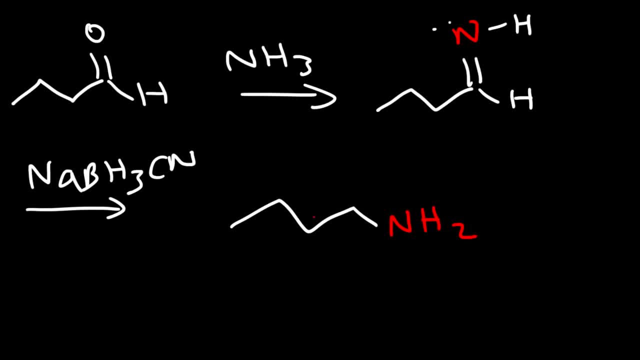 It's still a primary amine, but it's not on the middle of the chain, But rather it's on the end of the chain. Now we can also make secondary and tertiary amines, So let's start with a ketone. 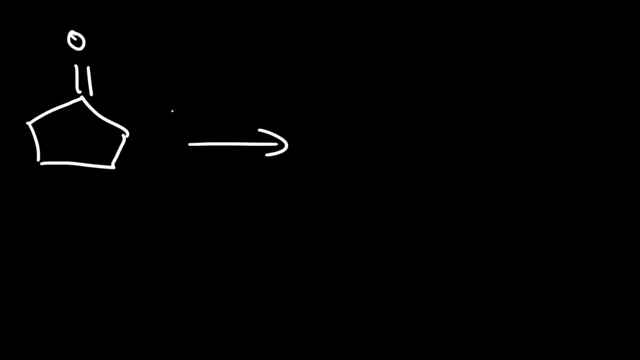 And we're going to react it with a primary amine, So we're going to lose water. If you take off the O and two hydrogen atoms, We'll get water as a side product, And so this amine has an R group attached to it. 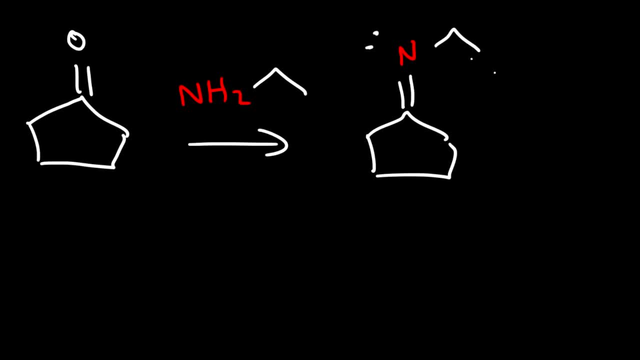 In this case an ethyl group, And now, once we reduce it with sodium cyanoborohydride, This is going to turn into a secondary amine. The double bond will be reduced into a single bond And we're still going to have the ethyl group attached to it. 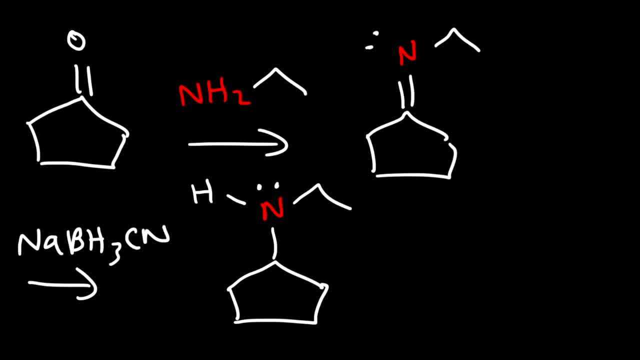 But now we're going to have a hydrogen and a lone pair. So that's how we can make a secondary amine: By using reductive amination, So to make the secondary amine React, the aldehyde or ketone, With a primary amine. 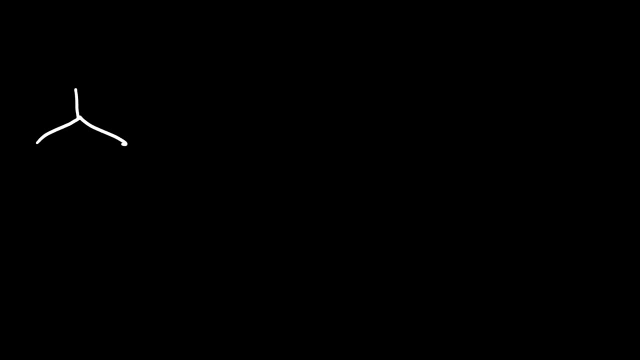 Now, if we want to make a tertiary amine Starting from a ketone, We need to react it with a secondary amine. So let's use diethyl amine And initially we're going to get the iminium ion, Which looks like this: 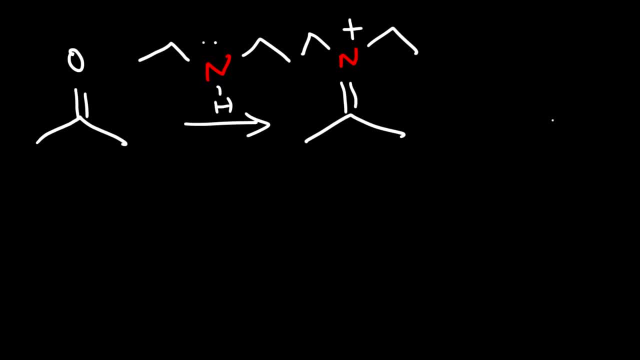 And this is an equilibrium with The enamine, So you may want to keep that in mind. So this is the enamine, But regardless of which form it's in, Once we add sodium cyanoborohydride, These two forms- 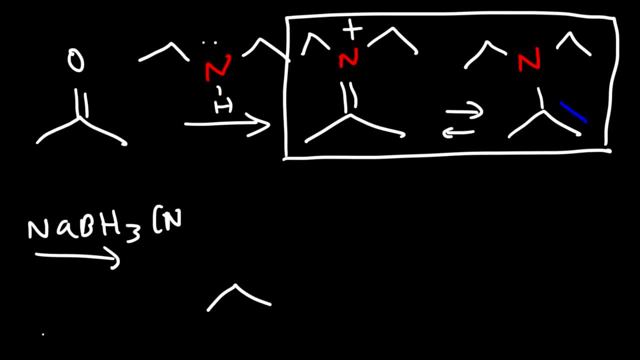 Will be reduced into a tertiary amine. So the double bond, Regardless of where it is, Is going to be reduced to a single bond. I'm going to need more space, So our final product will look like this. So this is how we could synthesize. 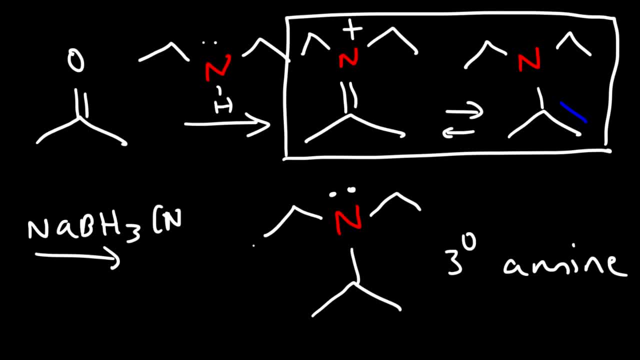 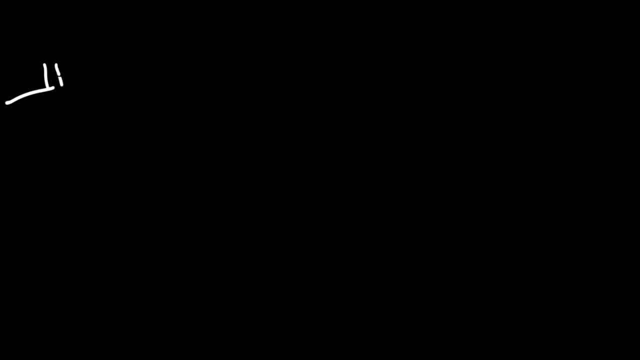 A tertiary amine. It's by reacting An aldehyde or ketone With a secondary amine. For the next reaction, Let's react an acid chloride With ammonia, But instead of writing NH3. I'm going to write it as HNH2.. 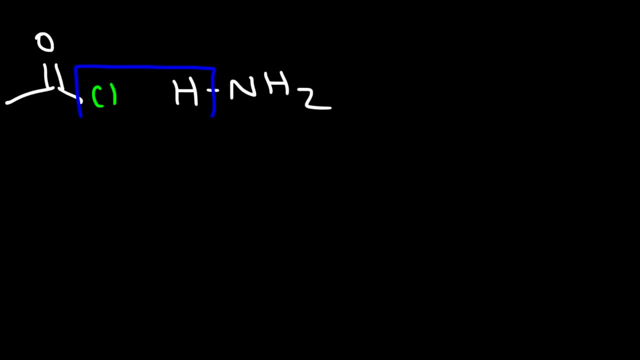 And so when you react an acid chloride with ammonia, You're going to get hydrochloric acid As a side product, So this will leave as a gas, And then for the other product You need to pair up these two together, And so an acid chloride with NH3. 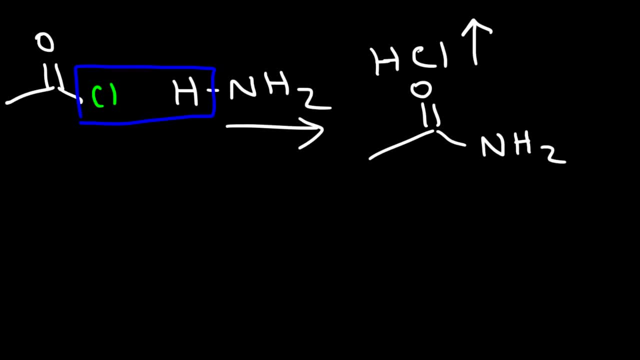 Will produce An amide. If you want to see the mechanism for this reaction, Check out the description section of this video. You could find My new organic chemistry playlist And in that playlist look for Carbosilic acid derivatives. 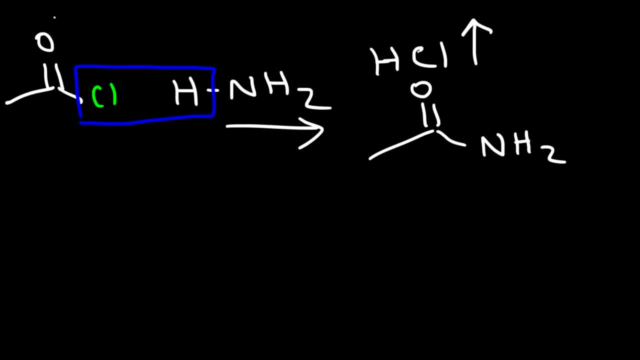 Those reactions. They have the mechanism where You can react an acid derivative with An amine or an alcohol or something else, But the mechanisms for those reactions are the same. So in this video I'm going to focus on The major product. 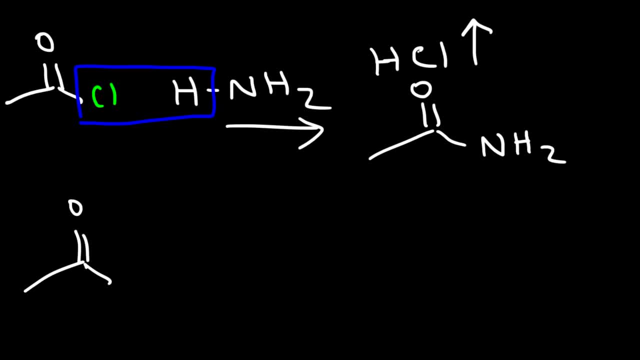 Now, once we have the amide, We could reduce this Into an amine, And so what we need to use at this point is Lithium, aluminum hydride, Followed by H2O, And so what's going to happen is. 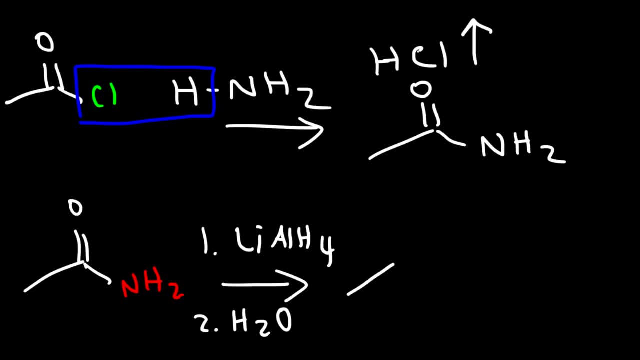 The carbonyl group is going to be reduced to a CH2 group, Converting the amide Into an amine. So that's another way in which we can make Amines. So this process is called acylation reduction. 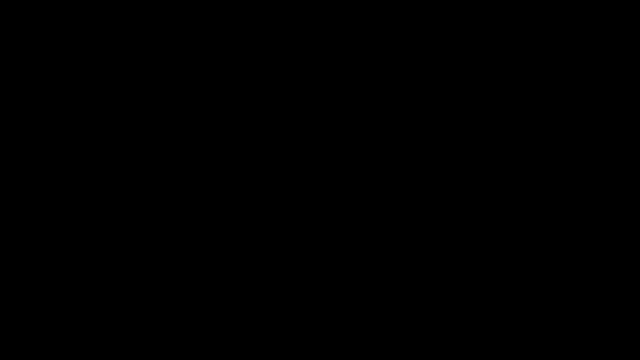 Now notice the pattern In these reactions. In the last example, We reacted in acid chloride with ammonia And we got a primary amine. So let's see what's going to happen If we react a primary amine With an acid chloride. 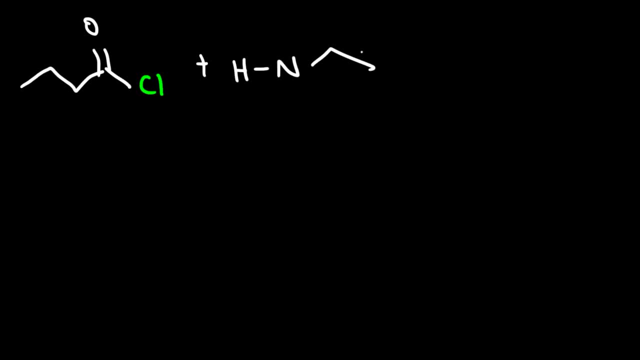 So this is going to be H? N With an R group. And here's the other hydrogen. So let's take out HCl as our side product, And so this will give us An amide With an ether group on it. 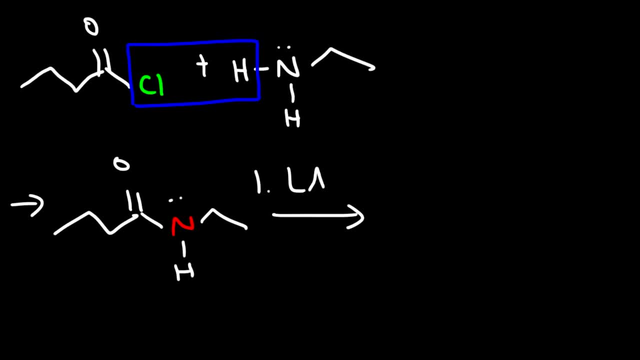 And then We're going to reduce it. Sometimes you might see lithium aluminum hydride Written like that, But if you do see that, It's the same, And so this carbonyl group Is going to convert into a CH2 group. 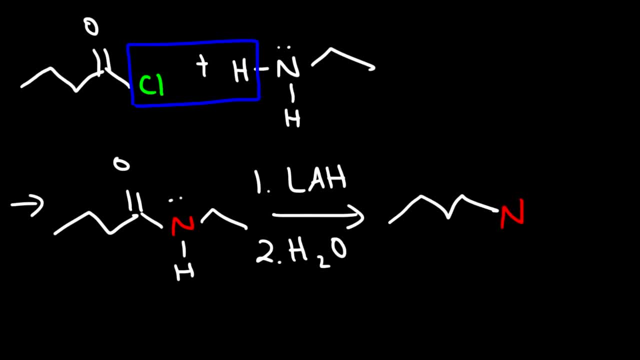 And so our product Will look like this. So the end result is that We have a secondary amine If we react to acid chloride with A primary amine, And the reason being is: We started with one R group, But we're going to add: 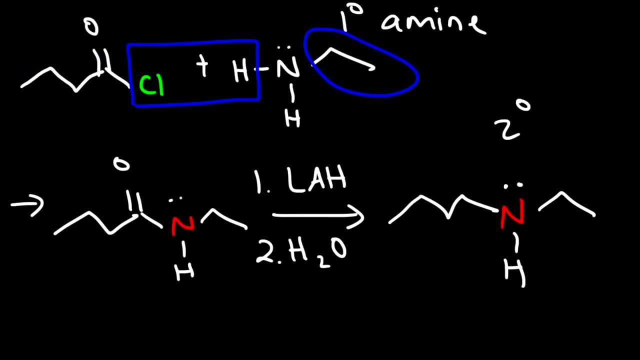 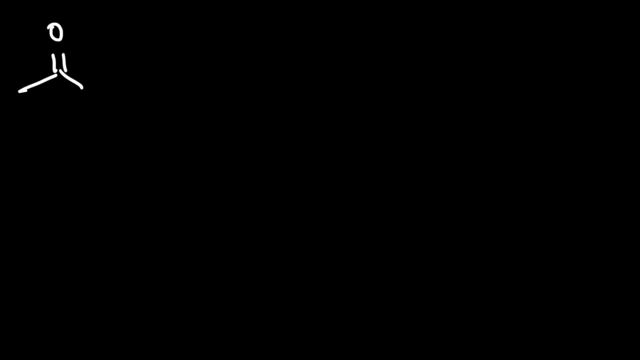 This R group to the nitrogen, So that's That's why it's going to be a secondary amine. Now, if we react The acid chloride With A secondary amine, You can guess what's going to happen. Eventually we're going to get a tertiary amine. 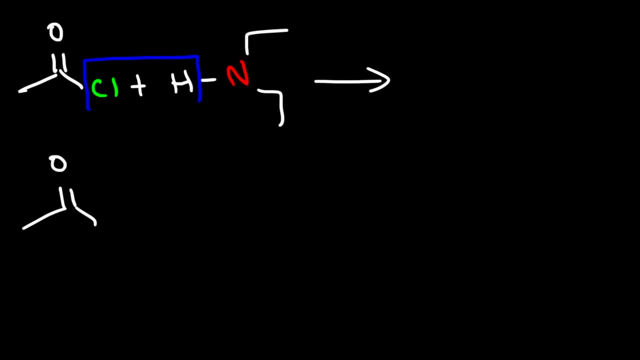 But first Let's take away hydrochloric acid And let's produce the amide, And then let's reduce it using Lithium, aluminum hydride, Followed by H2O, And so That's going to be reduced. 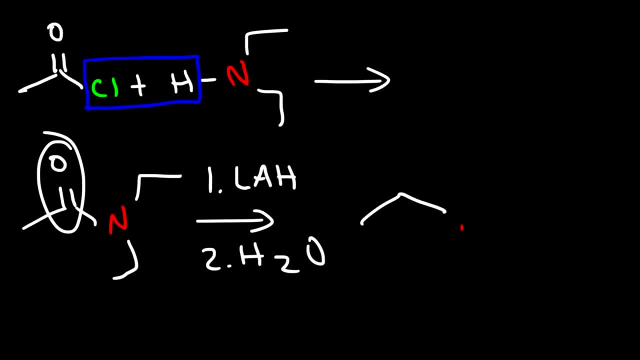 To a CH2.. And so this product is triethylamine. So you can make a tertiary amine If you react an acid chloride With A secondary amine Followed by Reduction. Now the next reaction we're going to talk about. 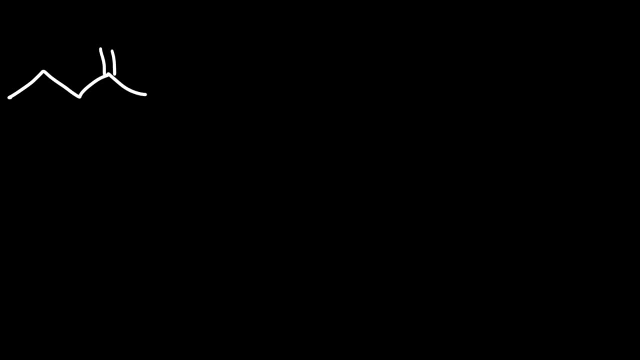 Is something called The Hoffman Rearrangement reaction, And so what we're going to do is We're going to react with a halogen. It could be BR2 or CL2.. Under basic conditions In water. And so what's going to happen is: 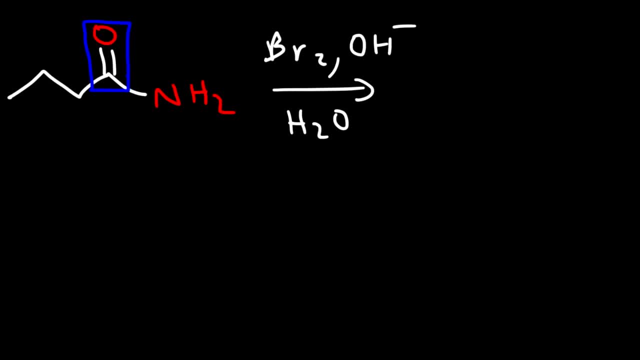 We're going to lose The carbonyl group. So we started with A total of Four carbons, But now we're going to have three carbons, And so this is going to be the end result Of this reaction. 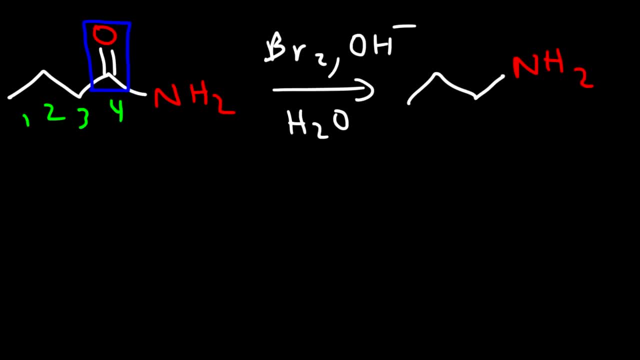 If you want to see the mechanism For this reaction, I have a separate video on YouTube. So if you just type in Hoffman, rearrangement, And then organic chemistry tutor, It should come up. Now the next reaction Which I also have. 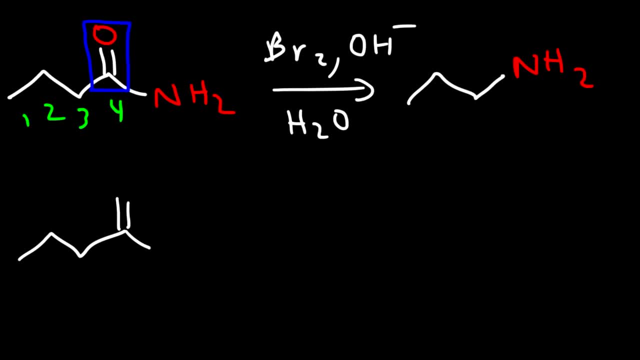 A mechanism for on YouTube Is called The Curtis Rearrangement, And so this reaction starts With an acid chloride, But instead of using These reagents, You're going to use Some azide, Followed by H2O. 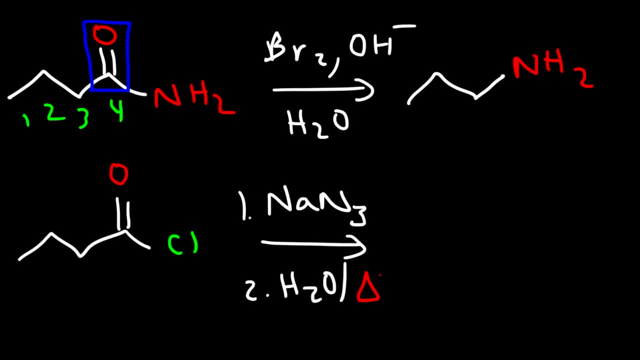 With heat. Now the effect will be Very similar. So we started with four carbons And we're going to have three, So we're going to lose The carbonyl group. The intermediate for this reaction Is an isocyanate. 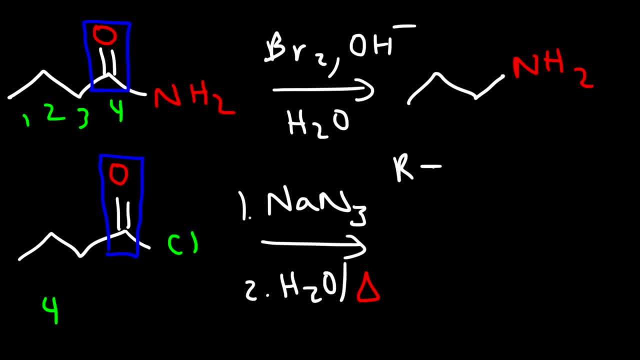 Intermediate. It looks something like this: It's an R group with an N Double bonded to a carbon Double bonded to an oxygen. But in that other video On YouTube that I have, You'll see how you can get that Isocyanate intermediate. 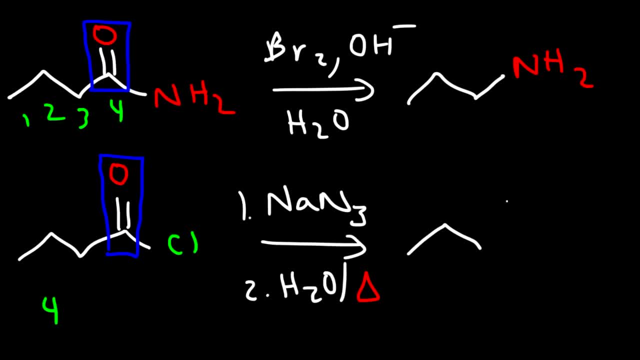 So once we lose this carbonyl group, We're going to have Three carbons And then the chlorine group We're also going to lose, But that's going to be replaced With an NH2 group Which comes from 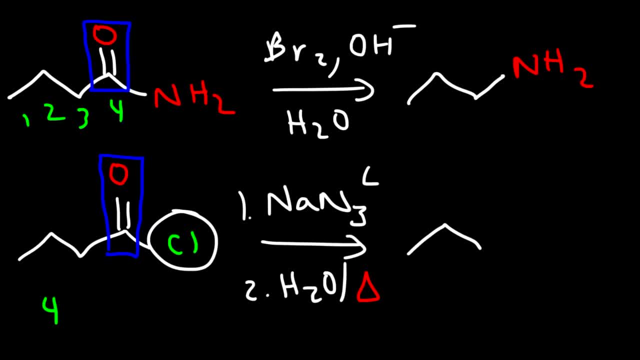 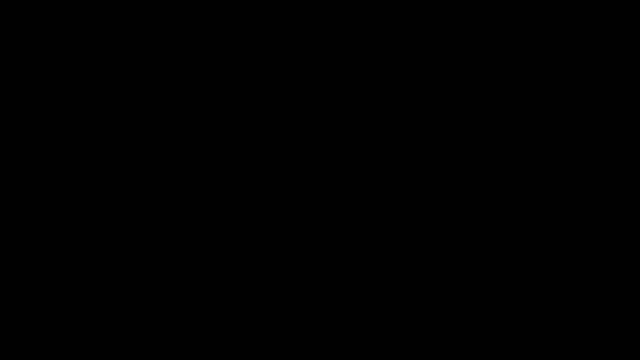 The N3. Minus azide ion. So the end result is that We're going to replace this entire Chloride group with an NH2 group, So we should have a total of Three carbons Instead of four. So let me give you some. 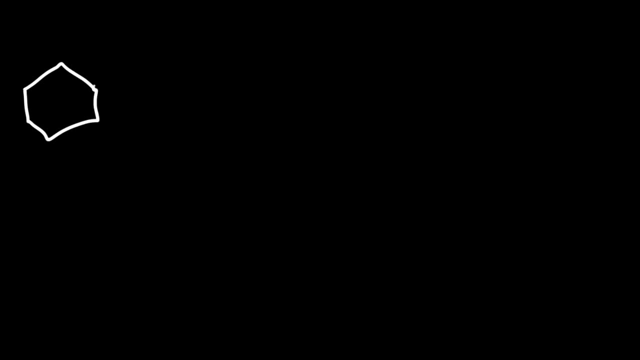 Example problems. So go ahead And draw the major product Of these two reactions. So here we have Cl2 with hydroxide And water, And for the second reaction, Here we have an acid chloride And we're going to react it with. 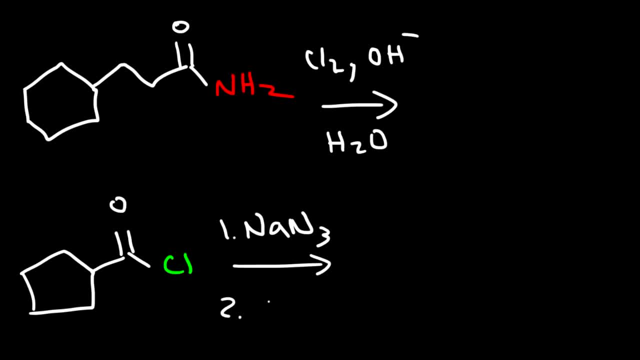 Sodium azide, Followed by H2O And heat. So the first reaction Is the Hoffman Rearrangement. All we need to do is get rid of The carbonyl group, And so we're going to have 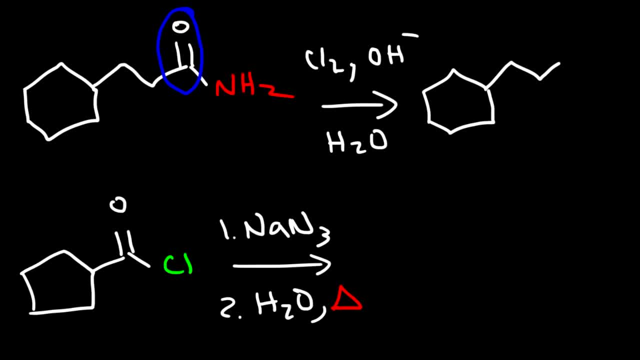 One less carbon. Everything else is going to be the same. So just to make sure, Let's count the carbons. So we have The six membered Cyclohexane ring And then these three additional carbons. So 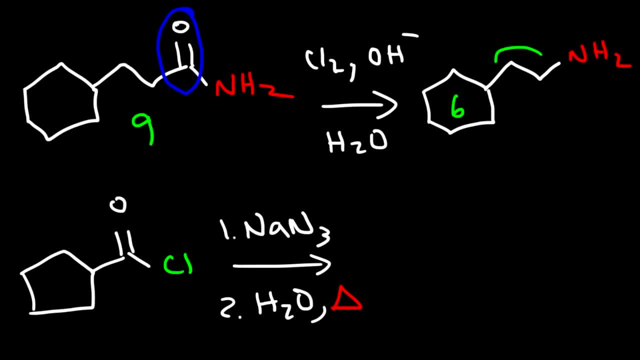 We started with nine carbons And now we have six Plus two, So we have a total of Eight carbons now. Now the next one is the Curtius rearrangement. So basically, what we're going to do is Take away this whole. 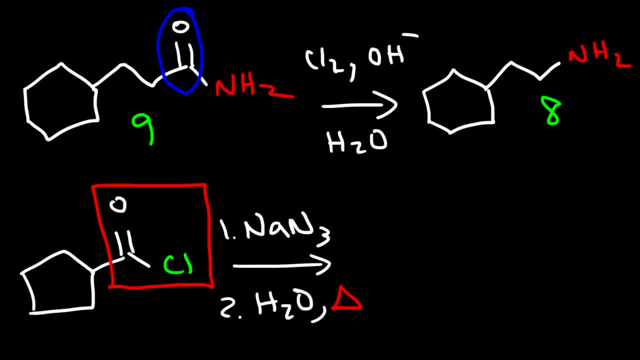 Entire Acid chloride group And just replace it With an NH2 group, And so that's going to be the end result For that reaction. Now, the next reaction that we're going to go over Is something called The Hoffman. 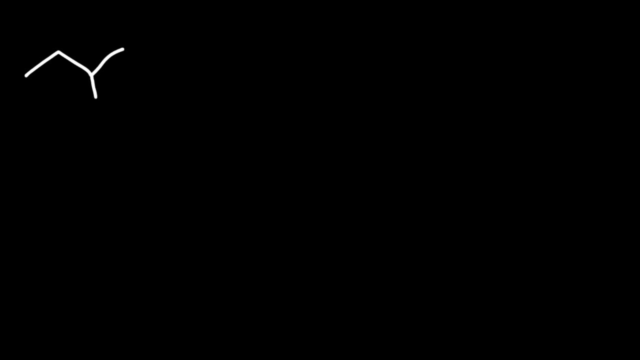 Elimination reaction, And so The overall process of this reaction is that It converts an amine Into An alkene, So it helps us to get rid of The NH2 group. That's on a carbon chain Or on a ring. 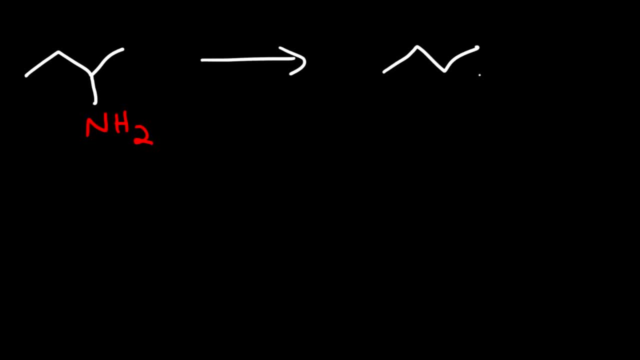 So what we're going to do Is we're going to Get rid of The H2O Rearrangement, And so We're going to Get rid of The H2O Rearrangement On a carbon chain. 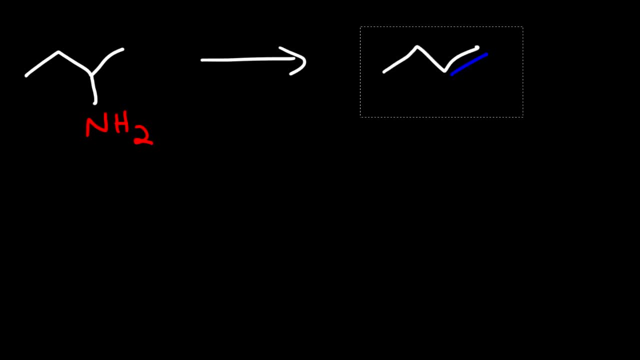 Or on a ring. So now The first step In this reaction, In the Hoffman Elimination reaction, Is to react The amine With Methyl iodide In excess. So we have to use Excess. 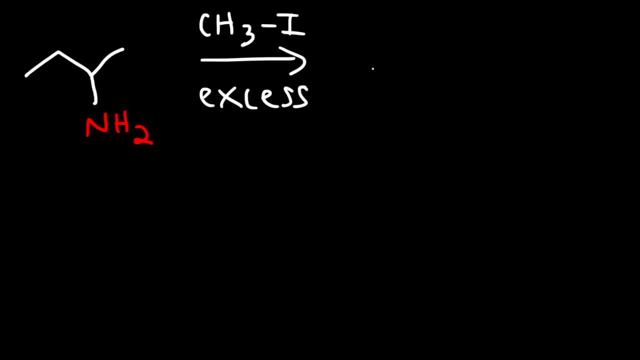 Methyl iodide, And so In a process Called Exhaustive Methylation, We're going to Add As many Methyl groups As we can To the nitrogen atom. So nitrogen Can only form Four bonds. 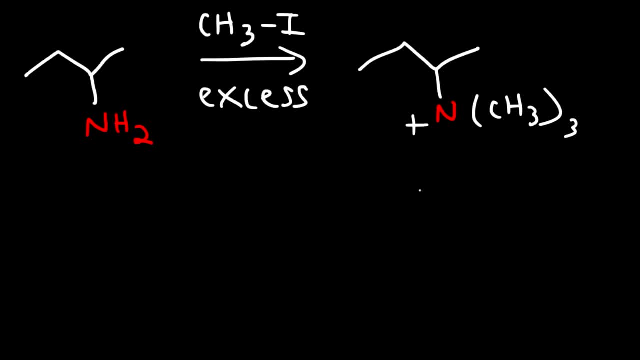 And when it has Four bonds, It's going to have A positive charge. Now We're also Going to have An iodide Ion In the solution. Now The next step Is to react It with. 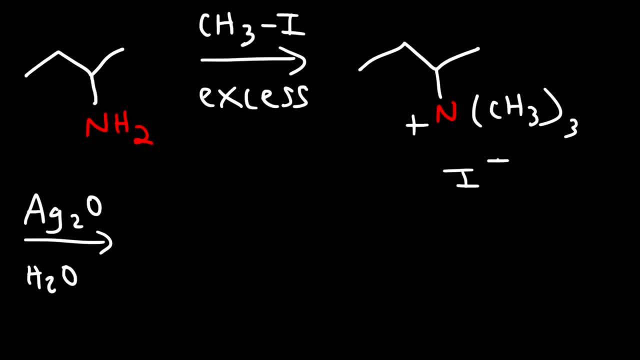 Silver oxide And Water. So what's Going to happen Is Iodide Has a strong Affinity For the silver Cation, It forms An insoluble Product Called Silver iodide. Now 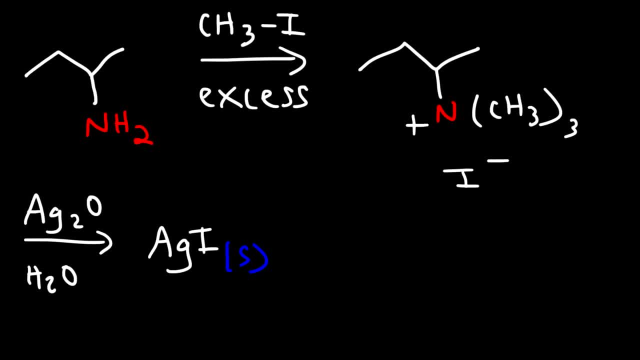 To displace The oxygen, And in water The oxide Will form Hydroxide, So the other Product Will be This product. We're still Going to have The quaternary Ammonium ion. 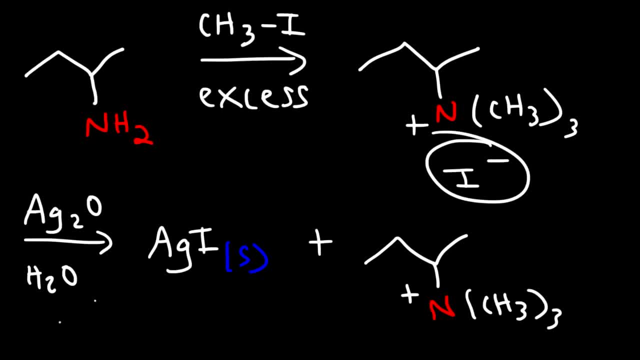 But Instead Of having Iodide As a free Ion, We now have Hydroxide In the solution. The purpose Of this Transformation Is to convert A bad Leaving group Into Neutral. 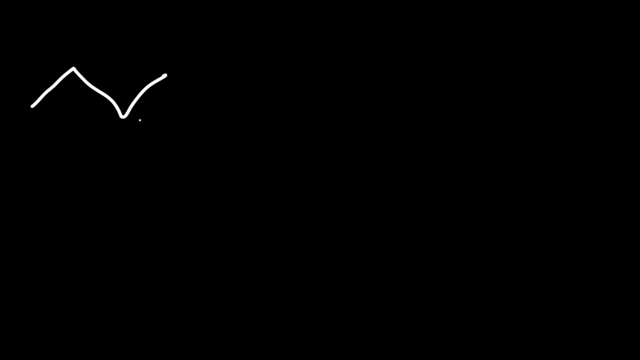 So once We have A better Leaving group, We can Now Perform Elimination Whenever The leaving Group Has A positive Charge. It's A better Leaving Group Than If It. 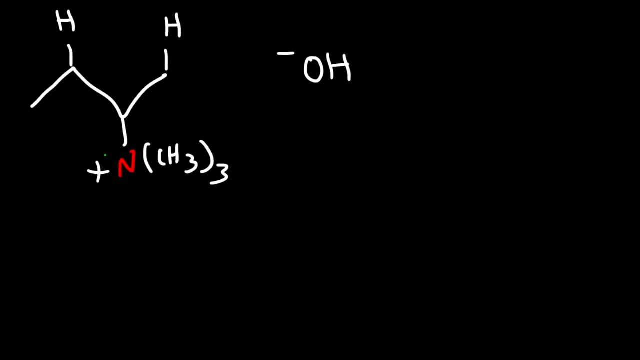 Was Neutral. Now We Have Hydroxide In. This Reaction Is Called The Hoffman Elimination Reaction, And Guess What It's Going To Give Us? The 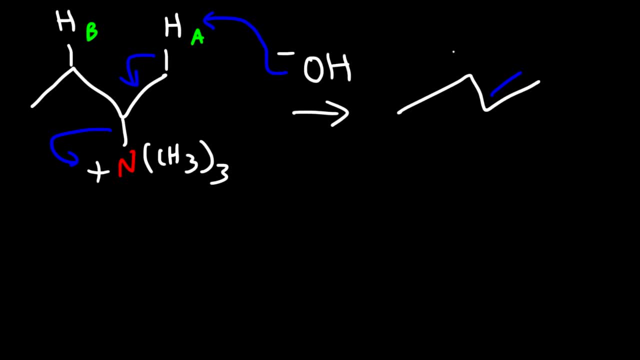 Hoffman Product, The Less Stable Alky. So Hydroxide Is Going To Go To Beauty, But These Two They Cost Into The Minor Product, Which 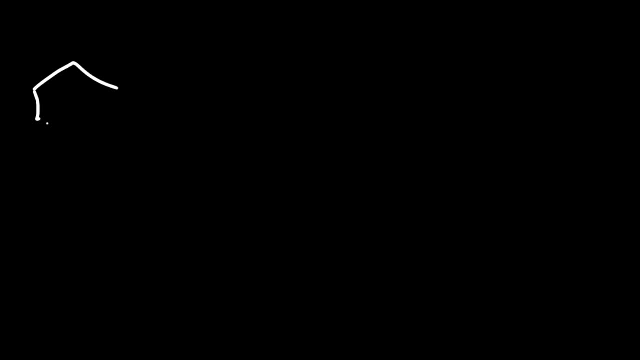 Is The Zeta Product In This Case, But Here The Major Product Is Going To Be The. So How Can We Completely Get Rid Of 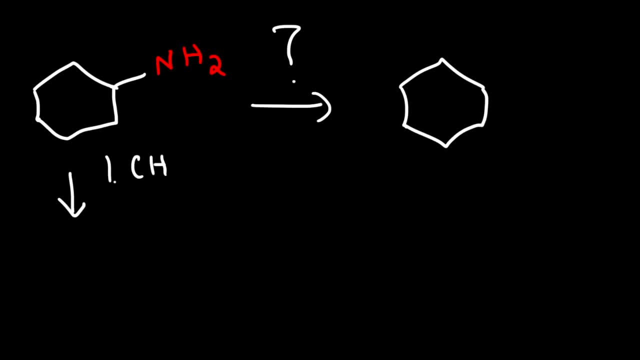 The H2. Group. What Reagents Do We Need Here? So The First Thing We Need To Do Is Perform The Hoffman. So We're Going. 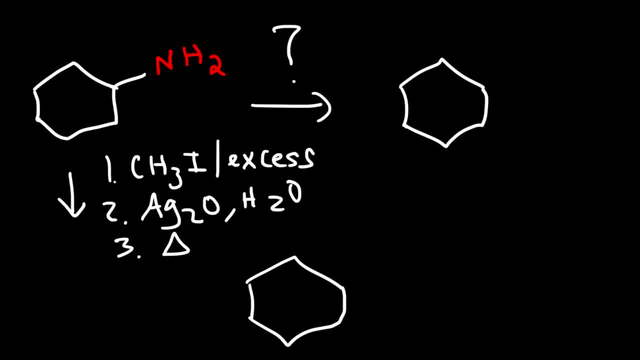 To Get This Now, The Last Thing We Need To Do Is Basically Hydrogenation, So We Can React This With Hydrogen Gas And A. 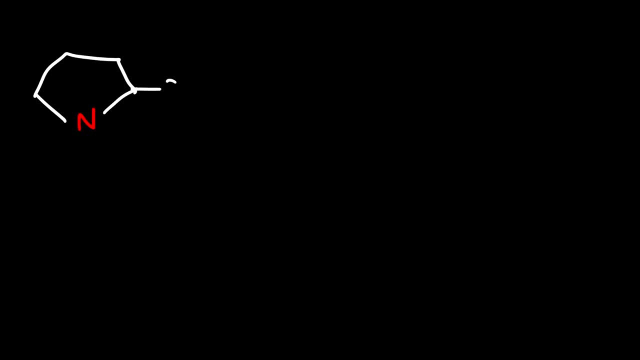 Palladium, Catalyst And Inside A Ring. What's Going To Happen If We Reacted With Excess Methyl Iodide Followed By Silver Oxide? 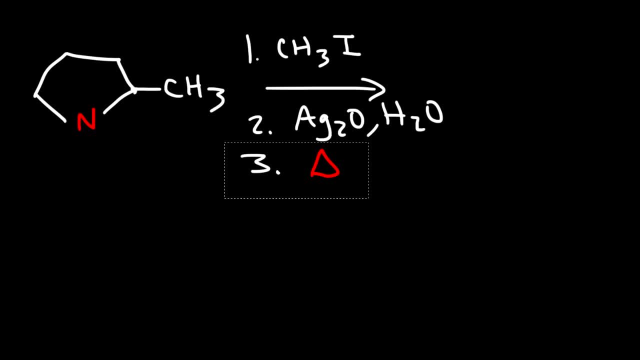 In Water, Followed By Heat. What's Going To Happen In This Reaction? The First Step Involves Methylation, So After Step One, We're. 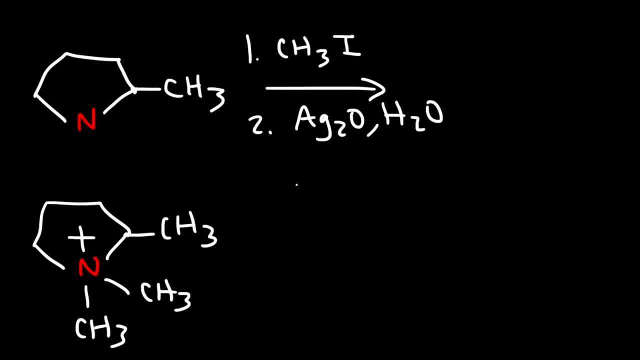 Going To Add As Many Methyl Groups As We Can To The Nitrogen Atom Until It Has A Positive Lead In. We're Going To 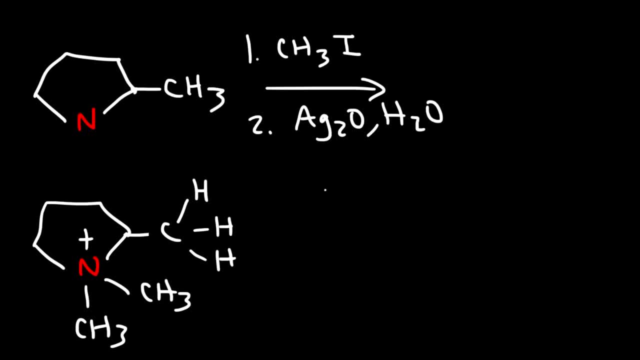 Form, An Alcheme. So Let Me Retry The Hydroxide Ion, And So The Base Is Going To Grab A Proton Form, A Double Bond. 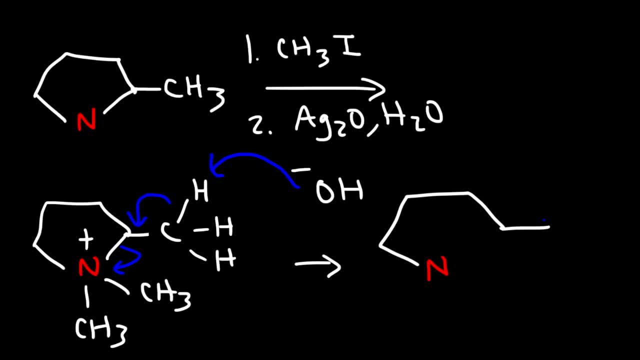 And Then A Carbon- Carbon Double Bond And We Still Have Two Methyl Groups On The Nitrogen Atom, So We Can Get A Mixture. 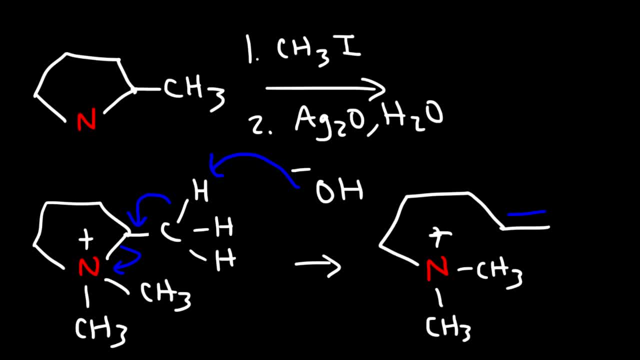 Of Products Here, But This Is A Nitrogen, And So We Get A Product That Looks Like This Right Now. The Nitrogen Shouldn't Have. 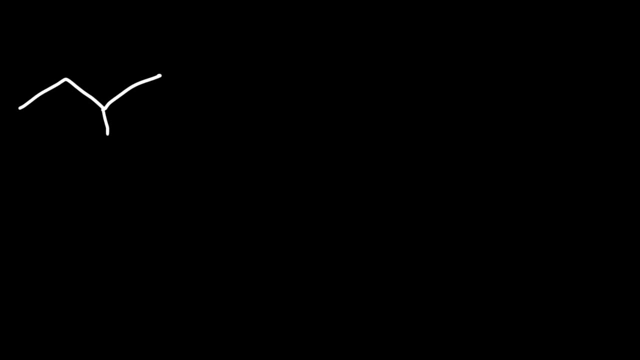 A Positive Charge Because It Has Three Bonds. Now It's Nitrogen. We're Only Going To Have Two Methyl Groups On It, So What We? 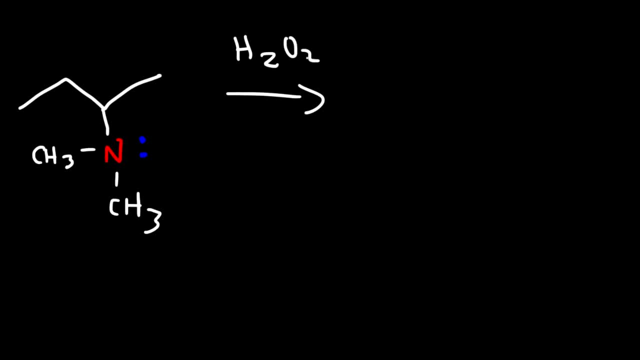 Have Is A Tertiary Amine As Opposed To A Quaternary Ammonium Ion, And Now We're Going On The Nitrogen, So At 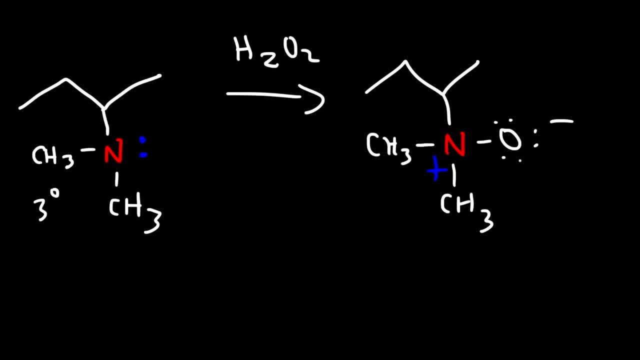 This Point: The Nitrogen Now Has Four Bonds, So It Has A Positive Charge. Now, Once We Heat The Solution, The Cope Elimination Will. 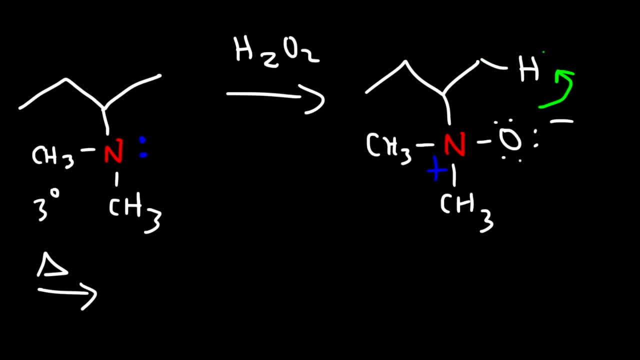 Occur In Stereochemistry. So It's Going To Go For The Hydrogen. The Carbon Hydrogen Bond Is Going To Break, Forming A Double Bond. 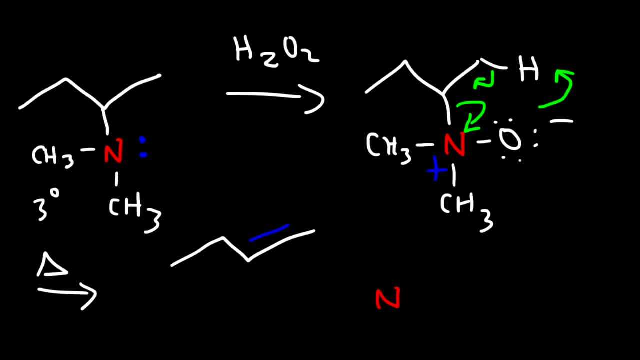 Kicking Out The Leaving Group, And So The End Result Is That We Still Get The Hoffman Product Over The Zeta Product As The Major. 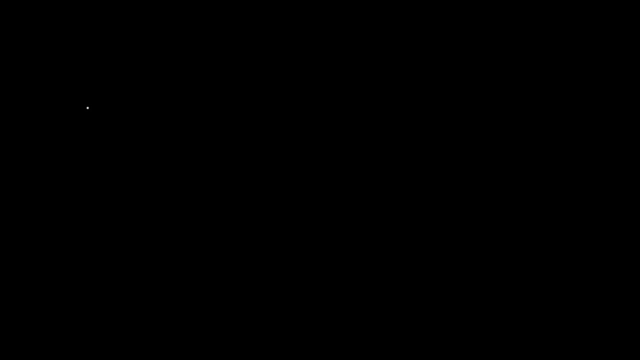 Product. So The Cope Elimination And The Hoffman Elimination They Have. So Here We Have Cyclohexanone And Here We Have An Alpha. 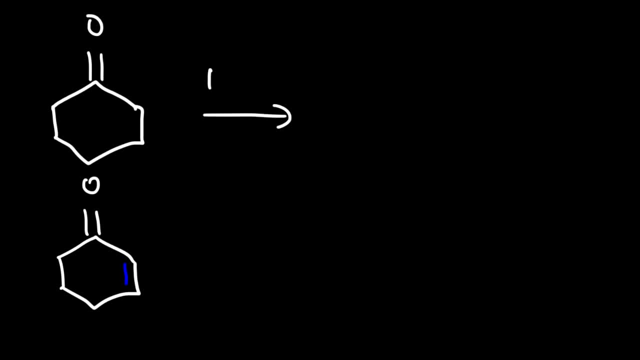 Beta Unsaturated Cyclic Ketone. So This Is The Alpha Carbon, This Is The Beta Carbon. What's Going To Happen? So The Nitrogen Atom. 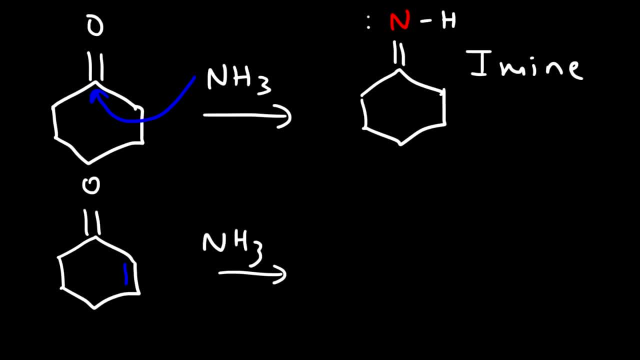 Will Attack The Carbon Group. Now, If We Have An Alpha Beta Unsaturated Ketone, The Nitrogen Atom Will Attack The Beta Carbon As Opposed. 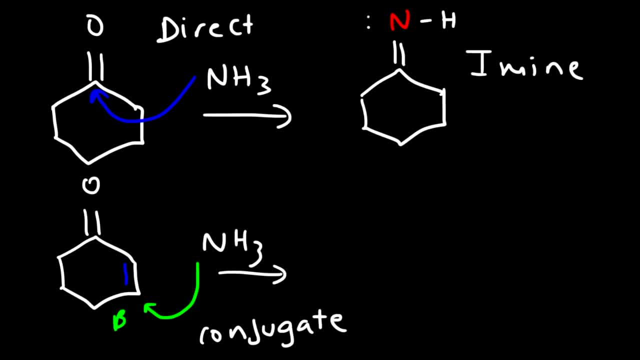 To The Carbon, No Carbon, And So We're Going To Get This Product Instead If We Have An Alpha, Beta, Unsaturated Ketone, So The